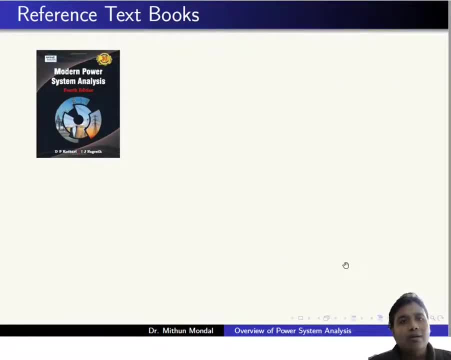 contents. So before that, let us see what are the reference textbooks that we are going to use for this particular subject. So one of the most important book of power system analysis is one by DP Kothari and IJ Nagarath. Second, you can follow power system analysis and design by: 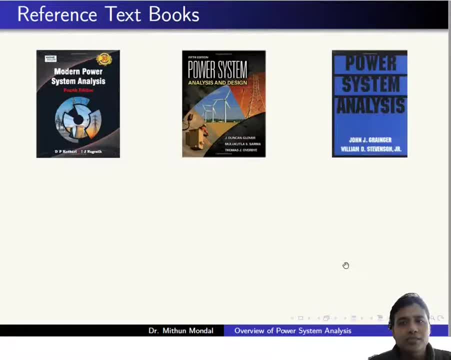 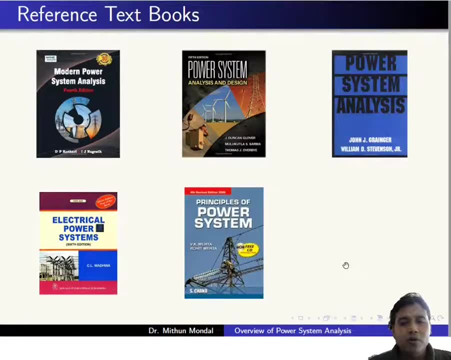 Duncan Glover. Power system analysis by John J Cranor. William D Stevenson. Electric power system by CL Wadhwa. Principle of power system by VK Mehta, Rohit Mehta. Power system analysis by JB Gupta. 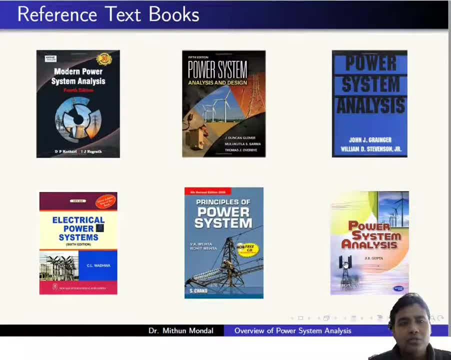 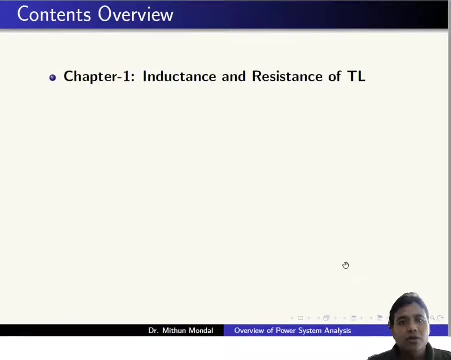 So these are few of the books, reference textbooks that you can follow for power system. There are other books also available which you can look into. So let us see the contents which we are going to discuss. So in the first chapter we are going to see the inductance and resistance. 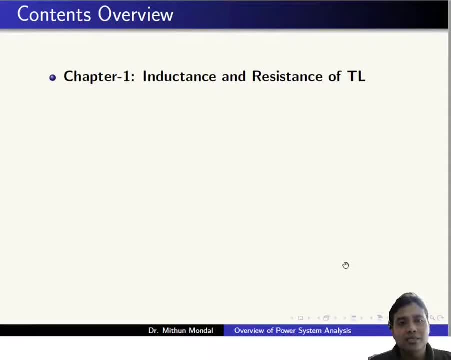 of transmission line. So I will be using TL as the short form for power system analysis. So inductance and resistance of the transmission line. Chapter 2 will be on capacitance of transmission lines. Chapter 3 will be on power system components and representation. Here the 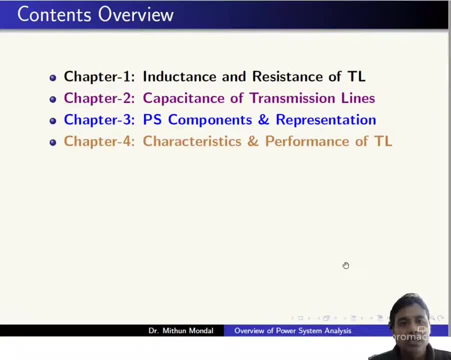 short form, TS, has been used for power system. Chapter 4 will be on characteristic and performance of transmission line. Chapter 5 will be on load flow studies. Chapter 6 will be on symmetrical fault analysis. Chapter 7 will be on symmetrical components. Chapter 8 will be on unsymmetrical fault analysis. 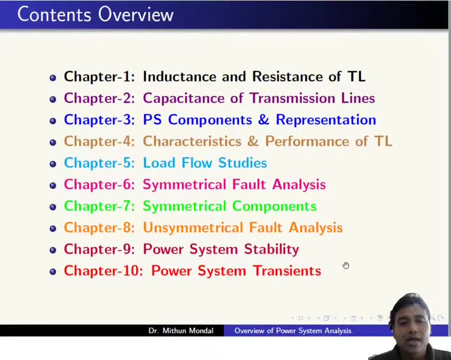 Chapter 9 will be on power system stability And chapter 10 will be on power system transients. So this is the overview of the 10 chapters that we are going to cover for this particular course, But before that we will be having two lecture series on the very basic fundamentals. 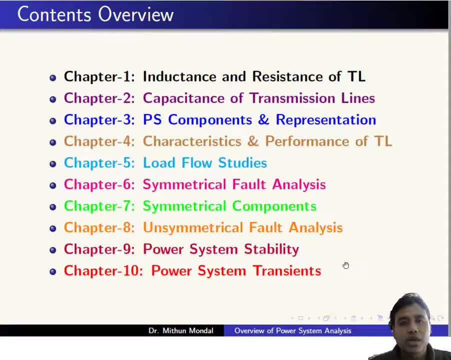 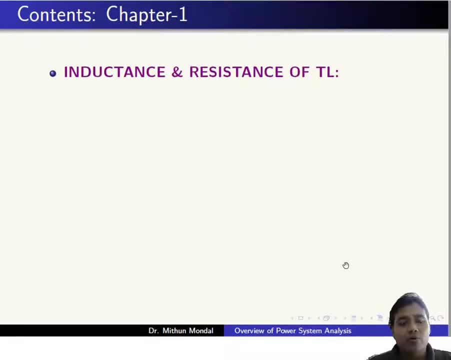 that we will be requiring to understand the course and you will discuss a little bit later. So let us see the contents one by one. The first chapter that I have said is inductance and resistance of the transmission lineSo here, the first, we will define what inductance. 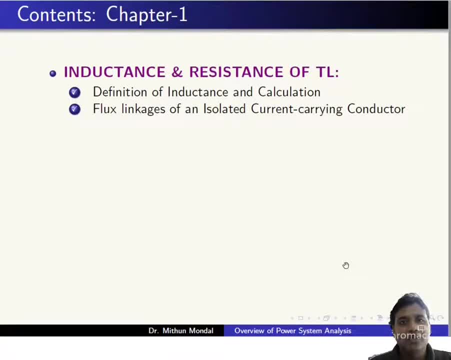 is all about and how do you calculate to find out the inductance? Next we will discuss. then we will discuss the inductance of a single phase two wire line. then we will discuss how many types of conductors are there for a transmission line. then we will discuss the flux linkage of. 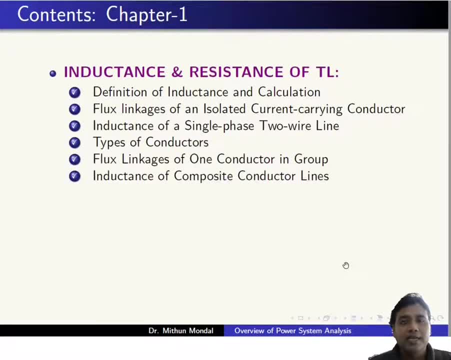 one conductor in a group of conductors. inductance of composite conductor lines. next we will be having inductance of the three phase lines. then we will have double circuit three phase lines. next we will discuss the bundle conductors. next we will discuss the resistance and its calculation. 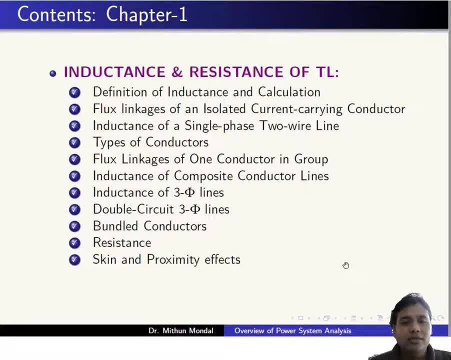 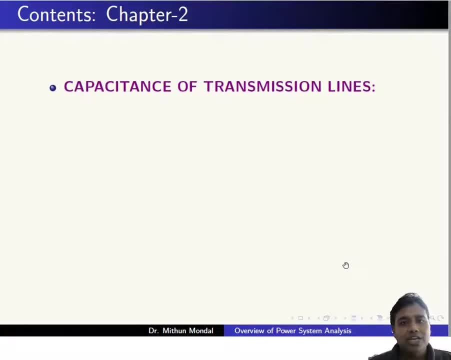 methods. we will discuss the method of skin and proximity magnetic field induction. so after covering chapter one, the next chapter will be on capacitance of the transmission lines which are the inductance of the three phase lines. then we will have double circuit, three phase lines, which covers the electric field of a long straight conductor. potential difference between two. 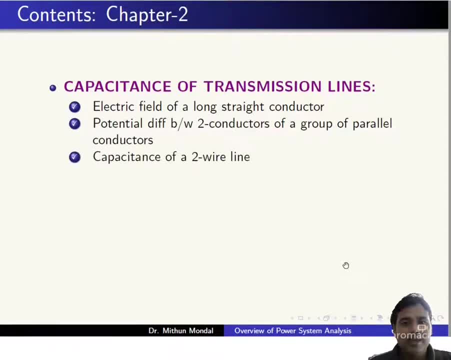 conductor of a group of parallel conductors. capacitance of a two wire line. capacitance of three phase line with equilateral spacing. capacitance of a three phase line with unsymmetrical spacing effect of earth on transmission line capacitance. then we will discuss the method of gmd, that is, geometric mean distance. 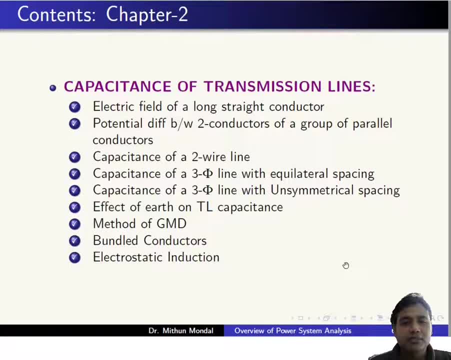 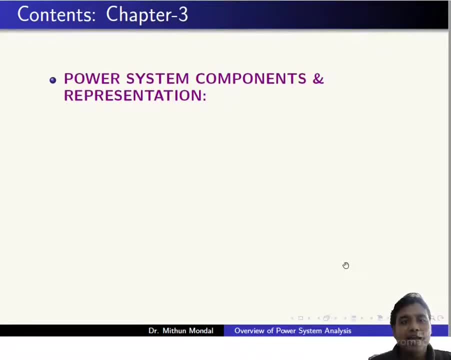 then we will discuss the bundle conductors and electrostatic induction. so these covers this chapter number two. next we will be having the chapter number three, so in chapter three is about power system components and representation, where the first will cover the single phase representation of a balanced three phase networks. next we will discuss this one line diagram, then we will discuss 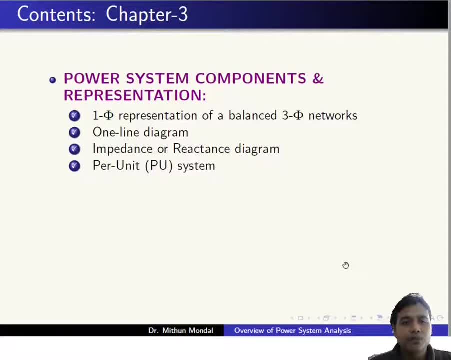 the impedance or reactance diagram. next we will discuss the pu system, which stands for per unit system. next we will discuss the complex power, the steady state model of a synchronous machine. next we will discuss the power transformer from the power system point of view: transmission of electric. 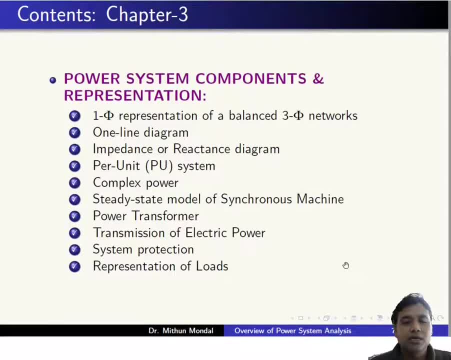 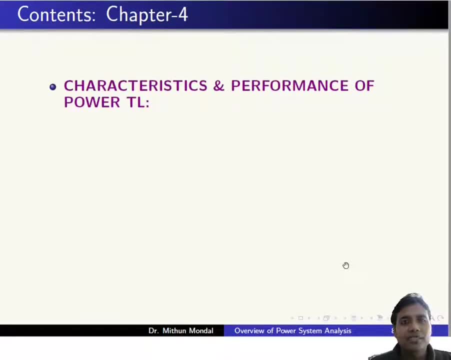 power system protection, representation of loads. this covers the chapter three. chapter four will be will be on characteristic and performance of power transmission line. So first we will discuss what is a short transmission line and its characteristic, medium transmission line and its performance, long transmission line and 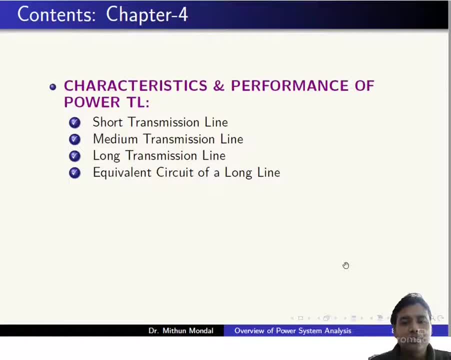 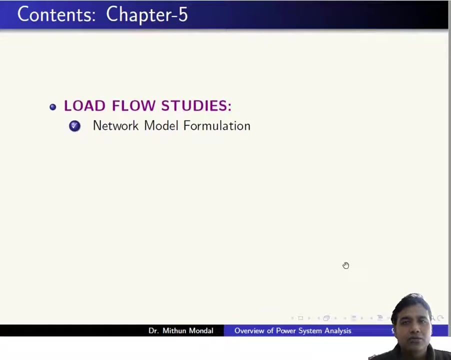 other modeling perspective equivalent circuit of a long line interpretation of the long line equations. current effect: tuned power lines. power flow through a transmission line. methods of voltage control. Next chapter that we have is chapter number 5, that is, on load flow studies. First we will discuss the network. 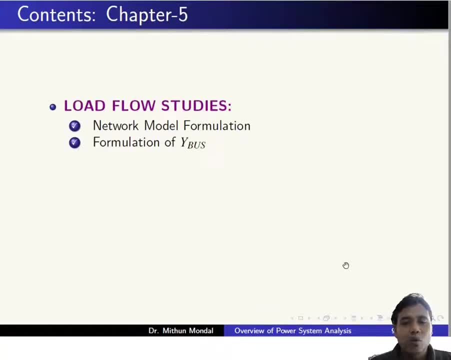 model formulation. formulation of Y bus load flow problem: Gauss-Seidel method, Newton-Raphson method, decoupled load flow studies. So these are the three methods- the Gauss-Seidel, Newton-Raphson and decoupled load flow- that will 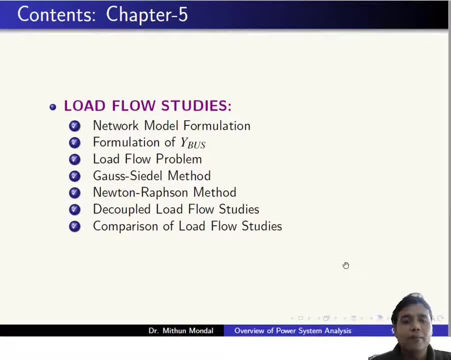 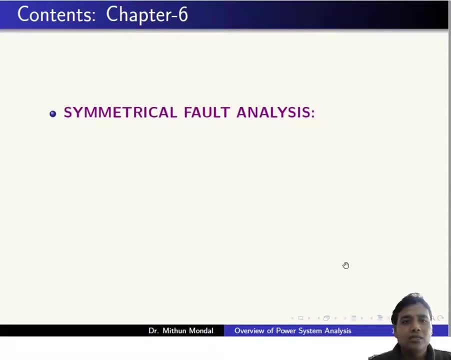 discuss under the load flow studies, and then we will compare all the three methods of the load flow. Next chapter we will be discussing is on symmetrical fault analysis. First we will discuss the transients on a transmission line: synchronous machine, short circuit on no load condition, short circuit of a loaded. 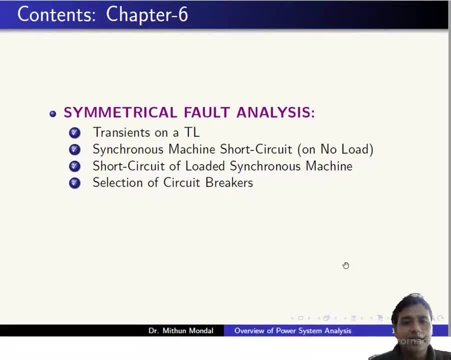 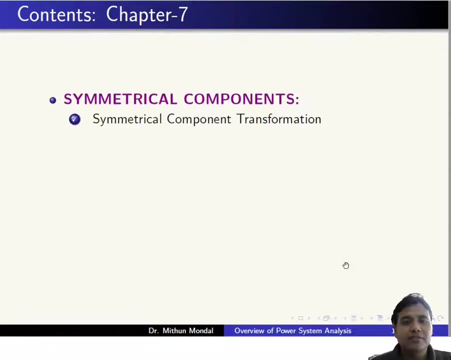 synchronous machine selection of circuit breakers. algorithm for short circuit services. direct level control outputed anxiety-tphen Tulip-Z bus functionality of заun Z bus formulations. Z stands for impedance here, so Z bus formulation. Next chapter we will discuss on symmetrical components, chapter number 7.. Symmetrical component. 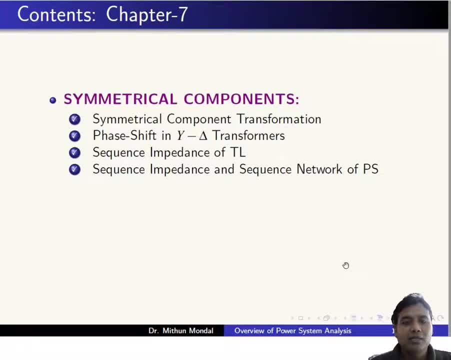 transformation: Facet, star, delta transformat. sequence impedance of transmission line. sequence impedance and sequence network of a power system. sequence impedance and network of a synchronous machine. The sequence impedance of transmission line. What I take waste are mystical components. fucking Kas McLean, Your jett celui해 cortígr Ahreats en. 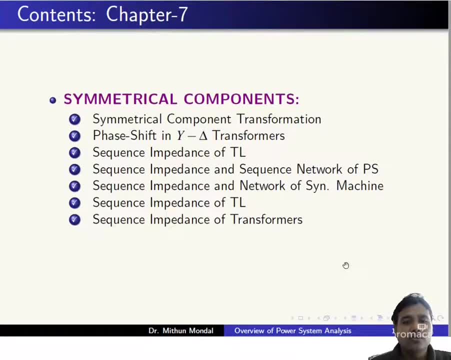 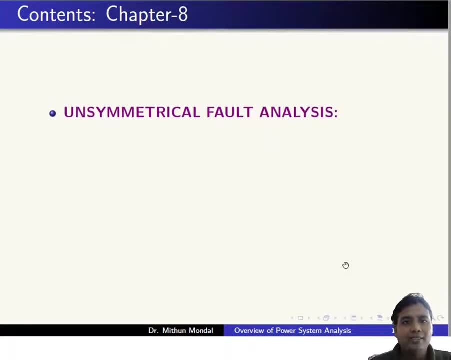 line sequence, impedance of transformers, construction of sequence network of power system. then we will be discussing chapter number eight, that is on unsymmetrical fault analysis, so symmetrical compound analysis of unsymmetrical faults. single line to ground fault, that is known as lg fault. line to line fault, known as ll fault. double line to ground fault that we say: 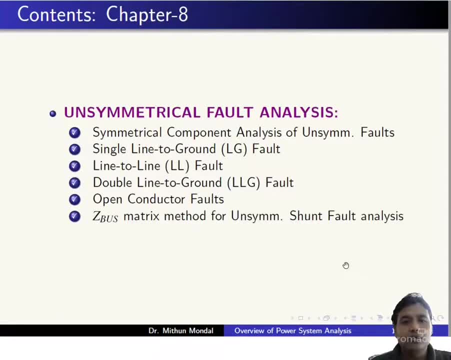 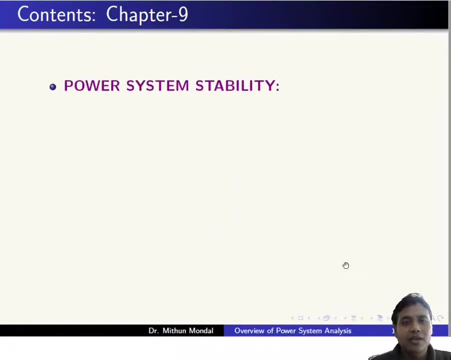 lg fault, open conductor faults, z-bus matrix method for unsymmetrical shunt fault analysis. then, chapter nine, we will discuss on power system stability. under power system stability we are going to discuss the dynamics of a synchronous line to ground fault known as lg fault. line to line fault, known as ll fault, double line to ground. 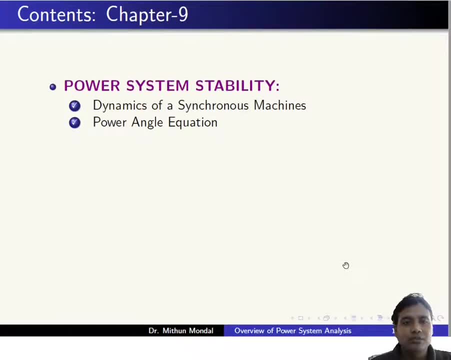 machine, the power angle equation, node elimination technique, simple systems. steady state stability, transient stability, equal area criterion, numerical solution of swing equation, multi-machine stability. what are the factors that affect the transient stability? the last chapter we will be discussing is power system transients, so here we will cover the types of system transients, traveling waves and 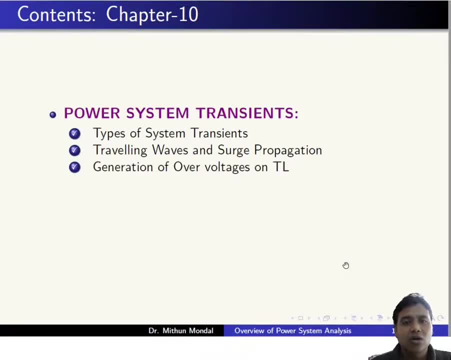 surge propagation, generation of over voltages on transmission line, protection of transmission line against lightning, protection of power system equipment against surges, insulation, coordination. so that completes the 10 chapters of power system analysis. next class and the succeeding class we will discuss the power system fundamentals. that is very important to understand this subject. 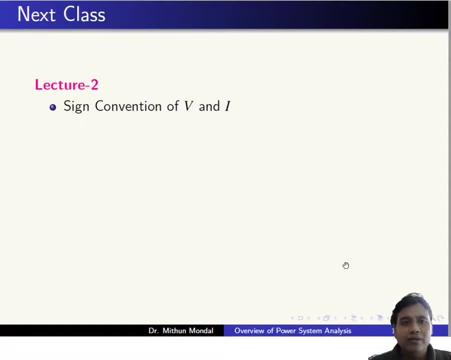 so lecture 2 will be the first part of the power system fundamentals. here we will first discuss the sign convention of voltage and the current. how do you represent the in terms of the phasor representation for the voltage and the current, conversion of time domain quantities, that is, the voltage and current, into phasors and then drawing?